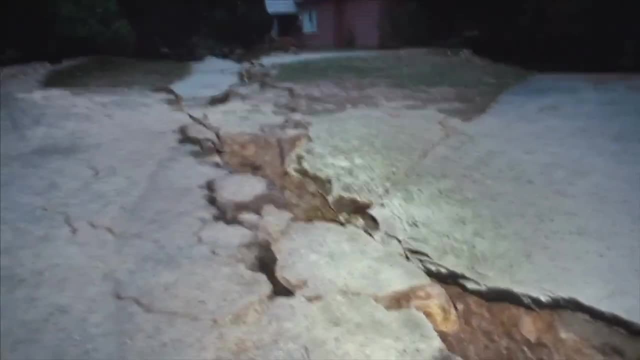 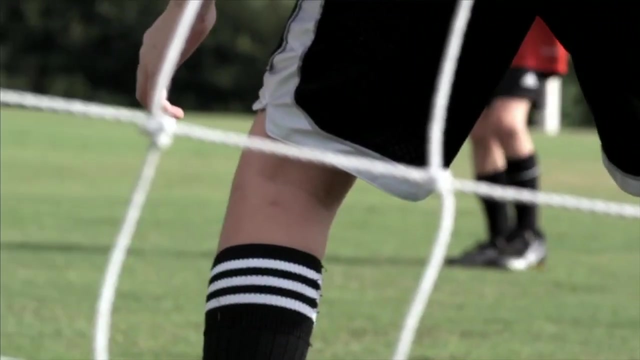 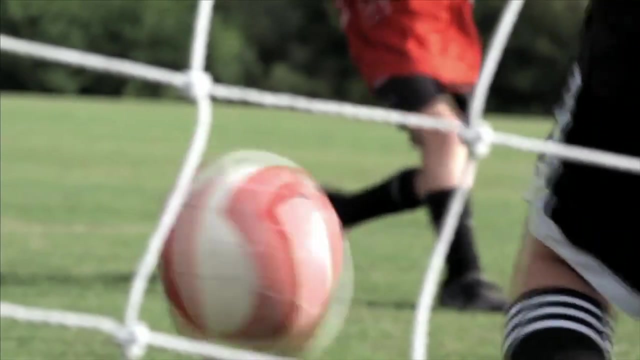 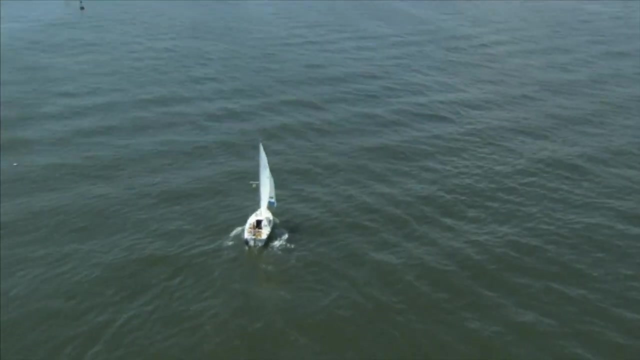 And then some that only move once in a great while. Motion is all about force. Force causes motion. A force is either a push or a pull. When a force pushes something, it pushes an object forward. It could make the object move faster. 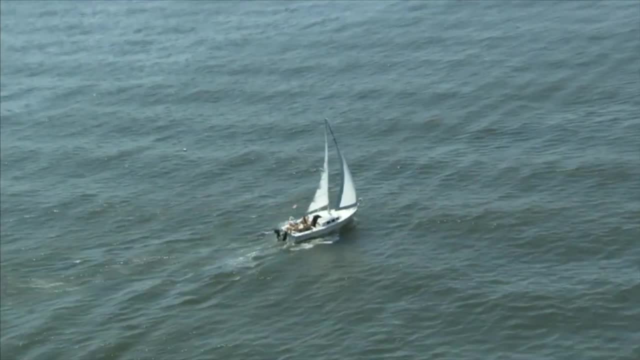 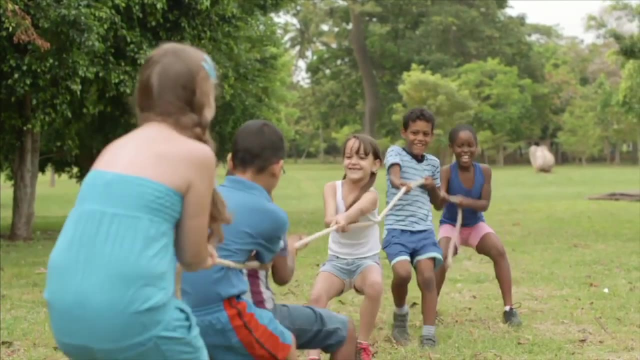 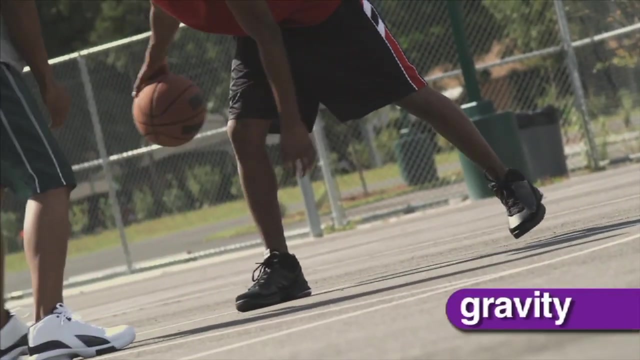 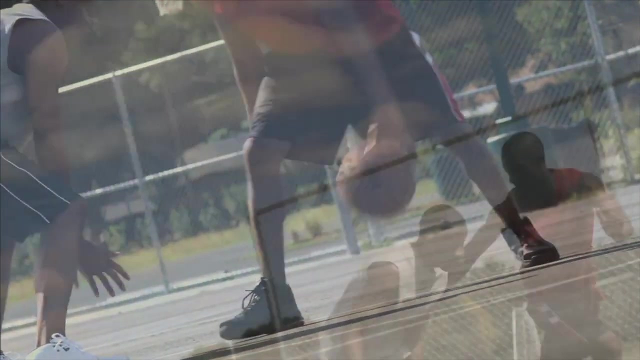 or move in a new direction. A force that pulls can make an object move slower or make it stop completely. Gravity is a force that pulls objects towards the Earth. When an object is dropped, it's the force of gravity that causes it to fall. 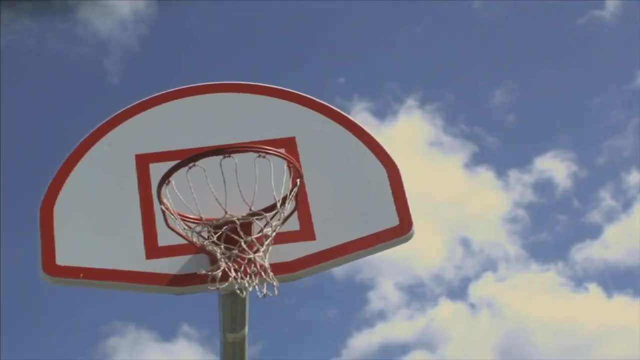 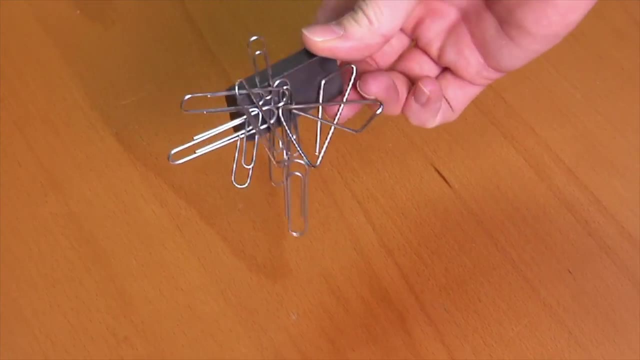 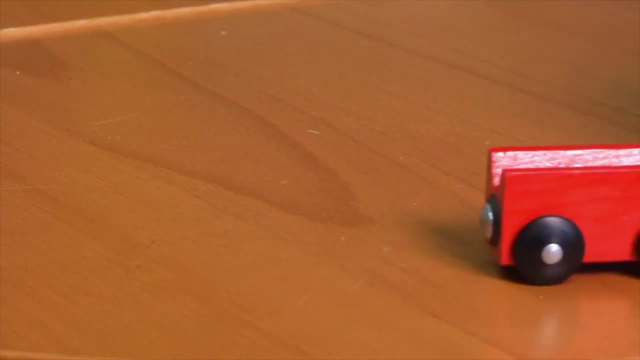 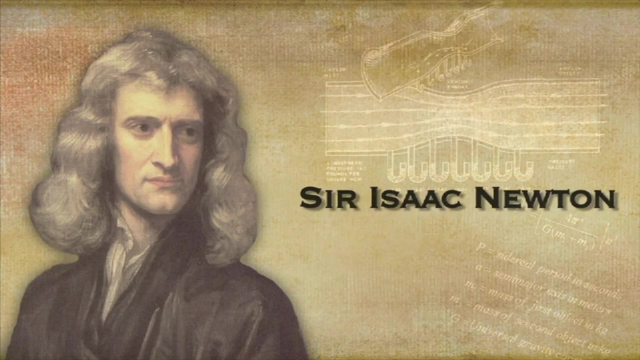 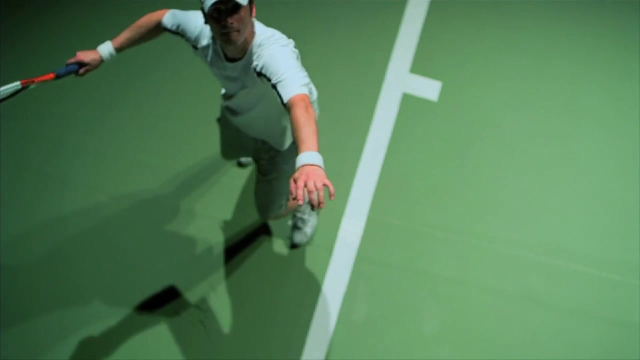 Magnetism is another kind of force. Magnetism is the property found in magnets. Magnetism can pull or push objects. Isaac Newton was a scientist who observed motion and created three laws of motion. Newton's first law of motion tells us that every movement or change of movement 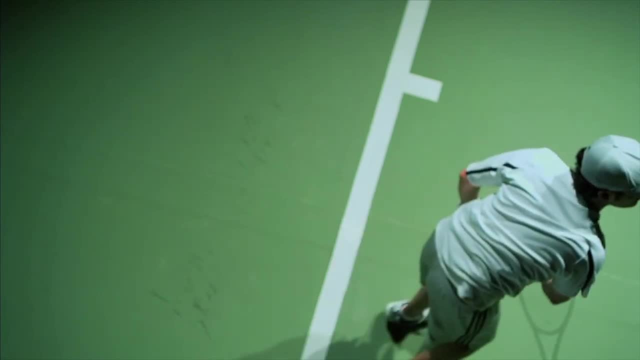 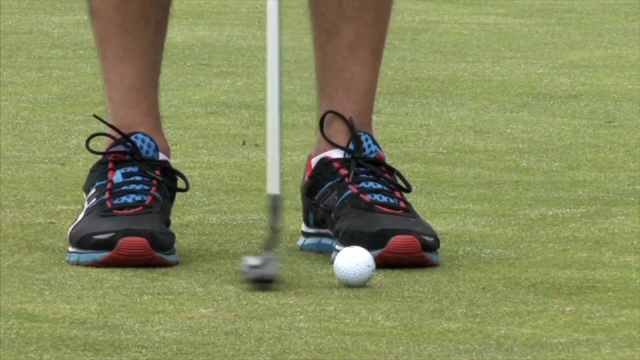 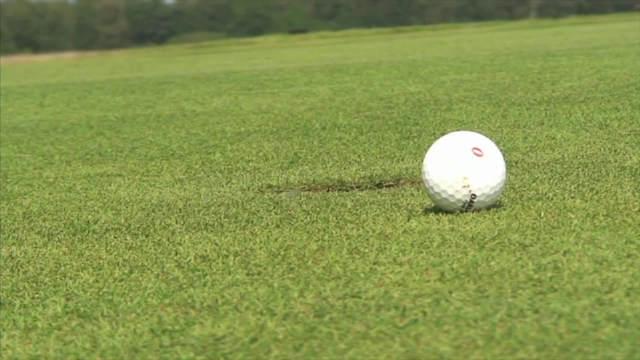 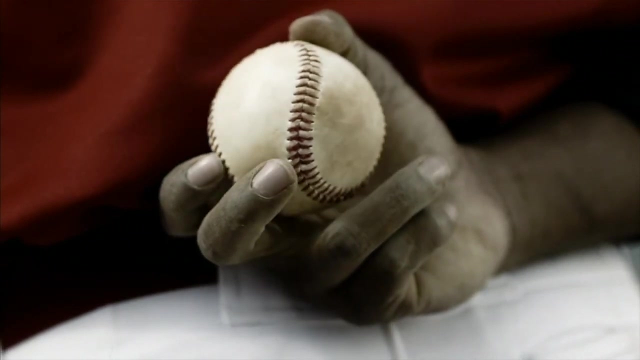 is the result of a force. For example, the force of a golf club causes the golf ball to roll, And when the ball stops rolling, it is a force that causes the ball to stop. Newton's second law of motion explains that the speed and direction of an object 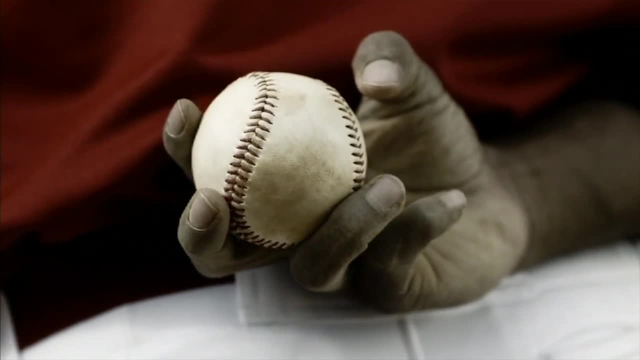 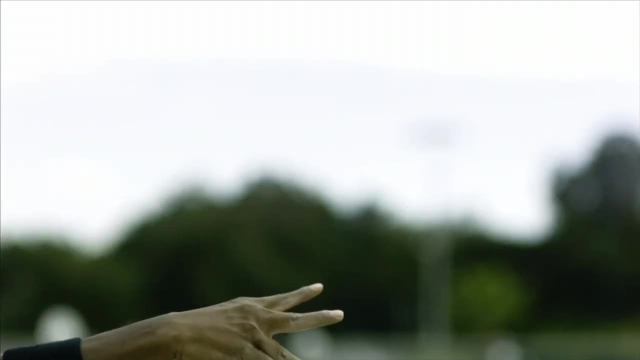 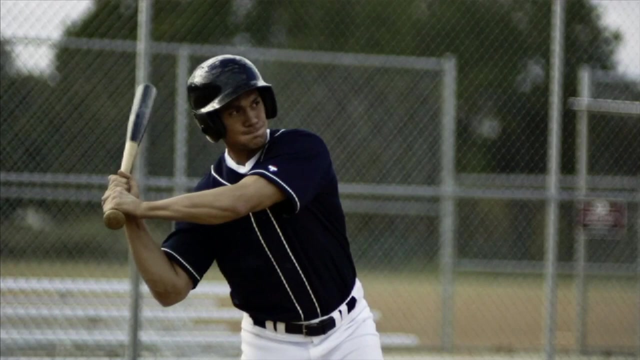 like this, baseball is determined by the force, how hard the pitcher throws and the mass of the ball. Newton's third law of motion explains that for every action the batter hitting the ball, there is a reaction. The ball flies off at a different speed and direction.